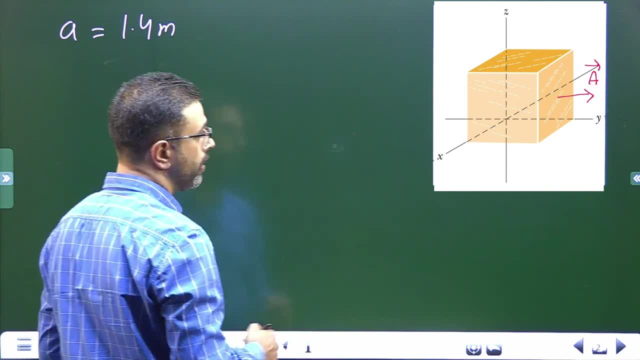 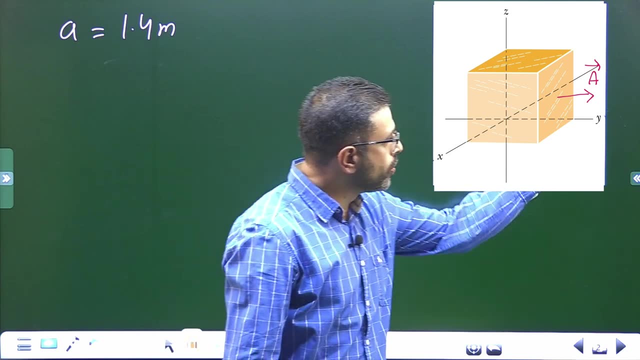 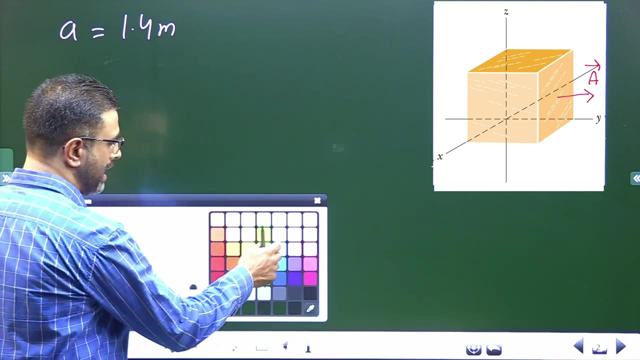 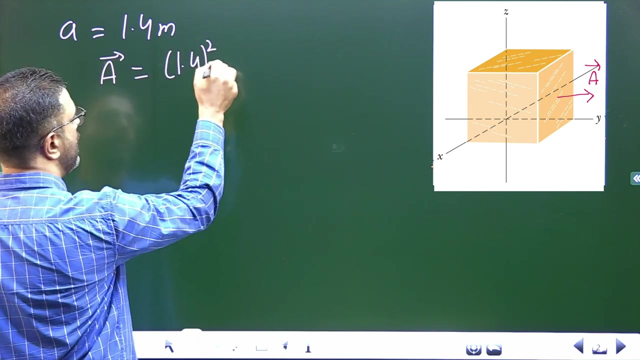 So first we are asked to find out flux through the right face. Right face is here, So direction of right face is this way. Now, this is the direction of right face, So that is in positive y direction. This is y axis, This is x here and this is z, So that is in positive y direction. So we can write area vector as 1.4 square side square into j. It is in positive y direction- into j. 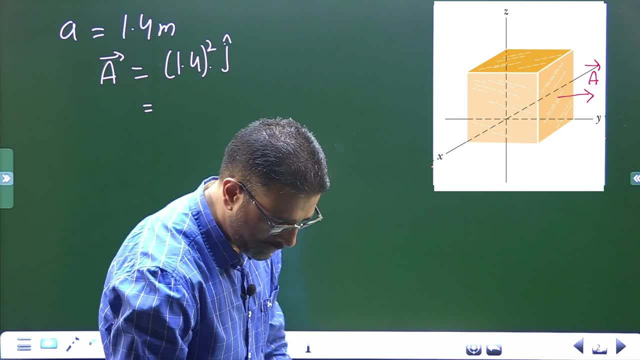 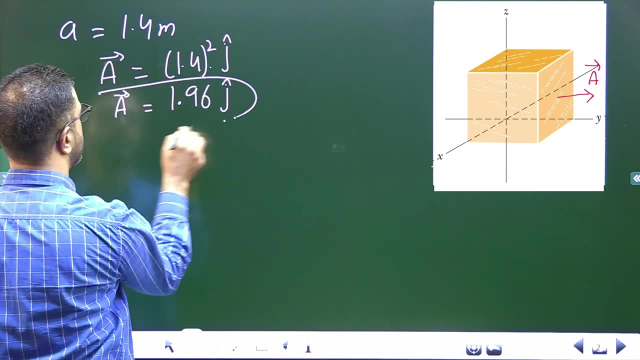 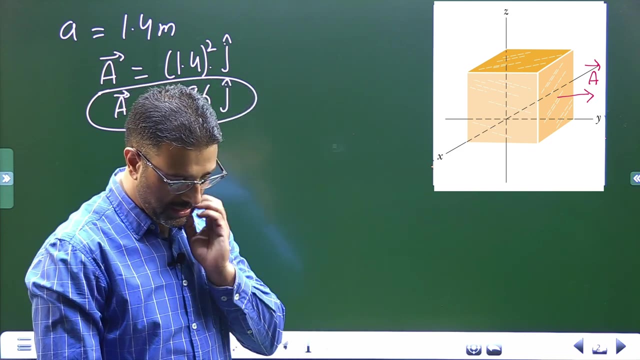 Now 1.4 square is 1.96, 1.96j. This is area vector. Then we have to find out flux through this one. In three cases fields are given. So part A, Let us go for part A. 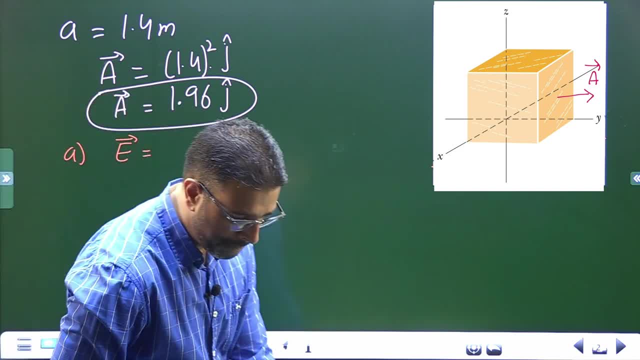 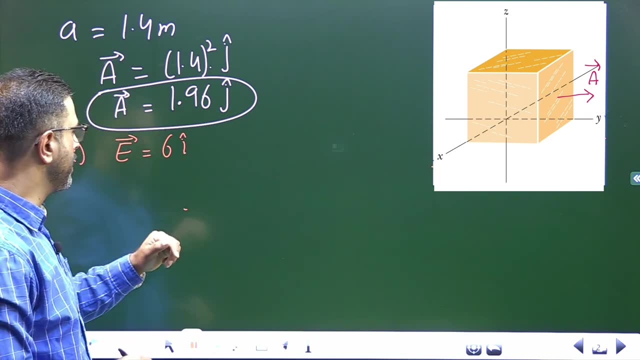 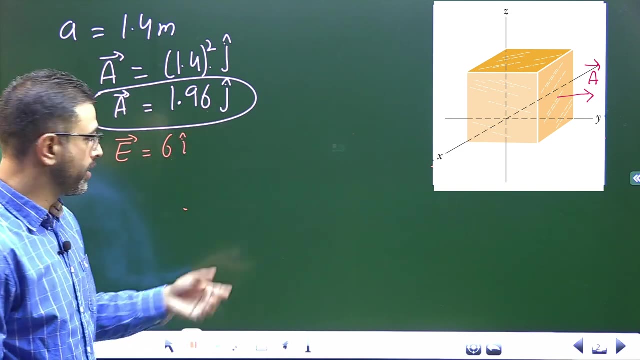 Part A. Field is given by 6i, Just 6i. So you can already see it is a constant, uniform field. It does not depend on any coordinate And it is in x direction. Field only has x component and area has only y component. So dot product is going to be 0.. 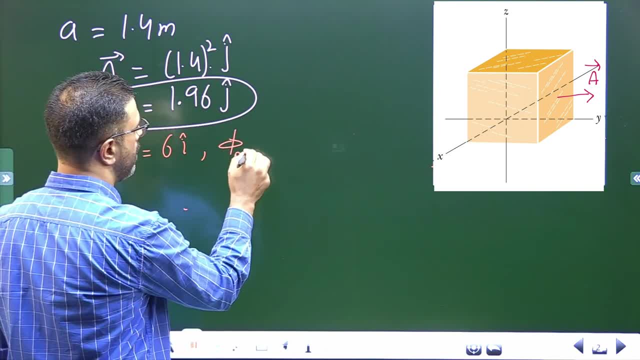 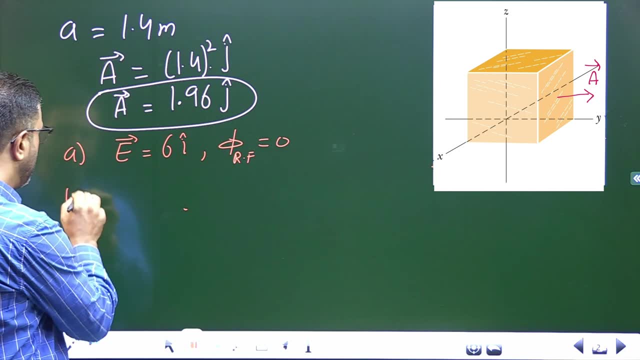 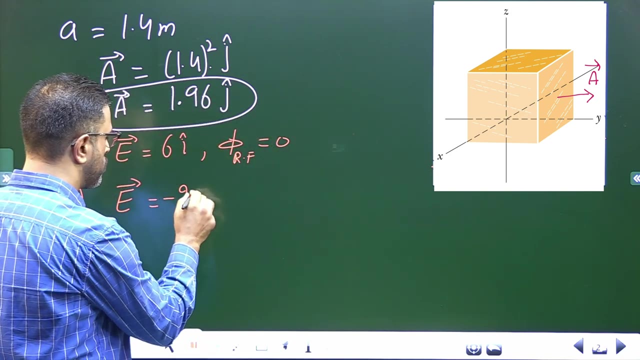 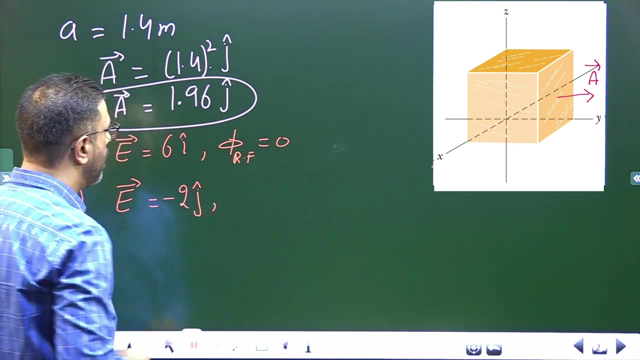 So flux through the right face, Right face, is 0, because one has only x component and the other has only y component. Then part B, Electric field, is given by minus 2j. Now area has y component and field also has y component. 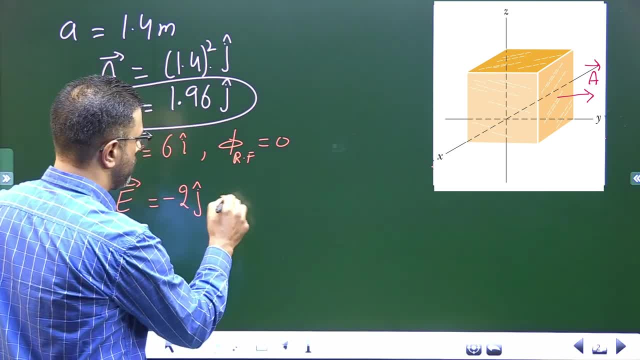 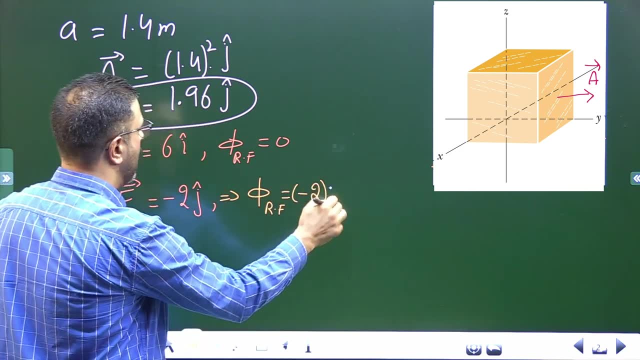 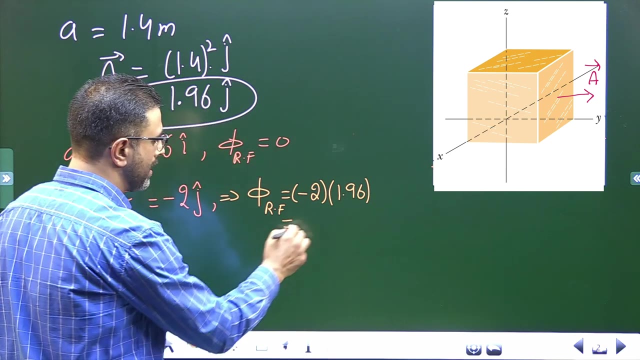 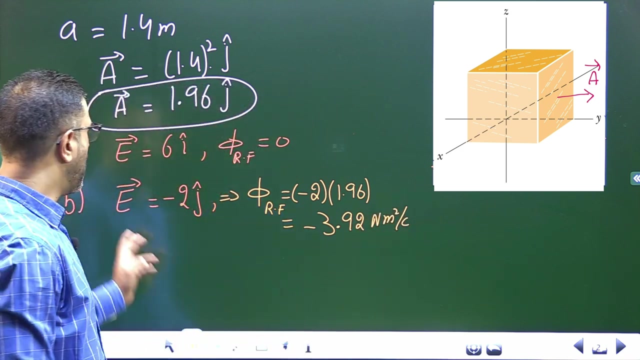 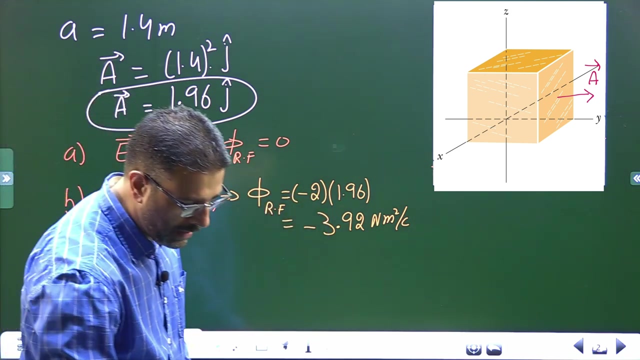 dot product will be non-zero. so this implies flux through the right face is equal to y component is minus 2 and y component is 1.96. that's equal to minus 3.92, minus 3.92 newton meter square per colon. so part b: we do have flux through the right face. then part c, then part c. part c: electric field. 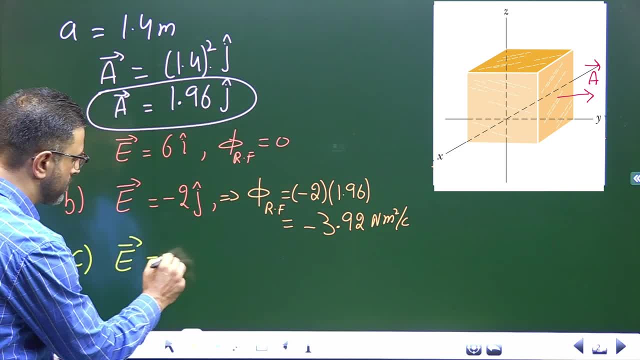 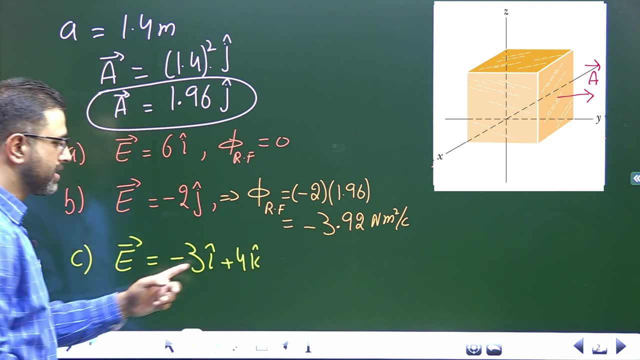 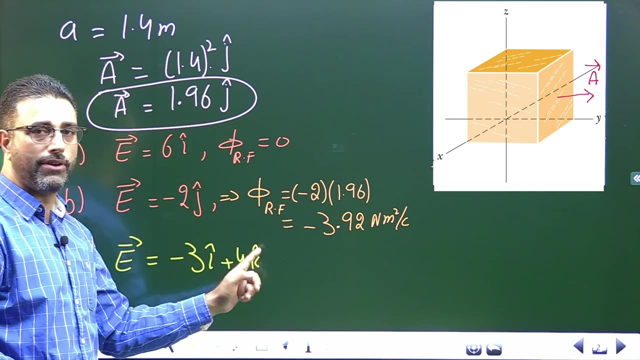 is given by minus 3i, electric field is minus 3i, and then plus 4k plus 4k. minus 3i plus 4k. okay, minus 3i plus 4k. now again you can see area has only y component and field does not have any y. 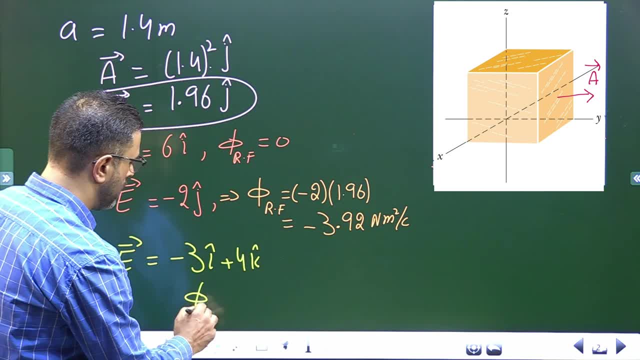 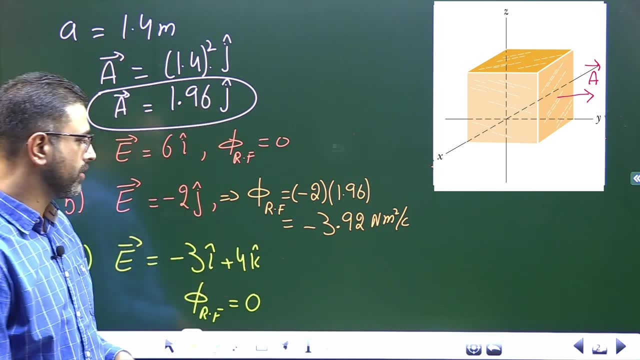 component. so dot product will be non-zero. so this implies flux through the right face is equal to zero. so flux through the right face in this particular situation is zero. this has only y component and this does not have any y component, so flux. now then we are asked to find out total. 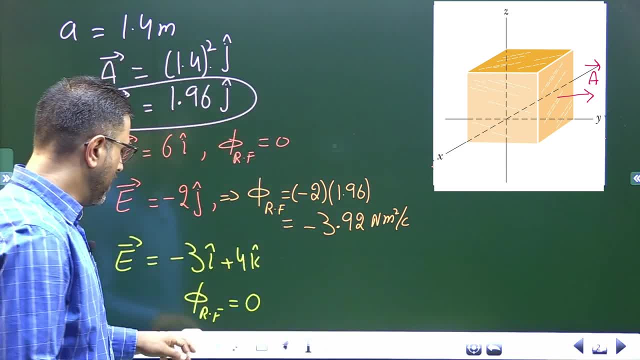 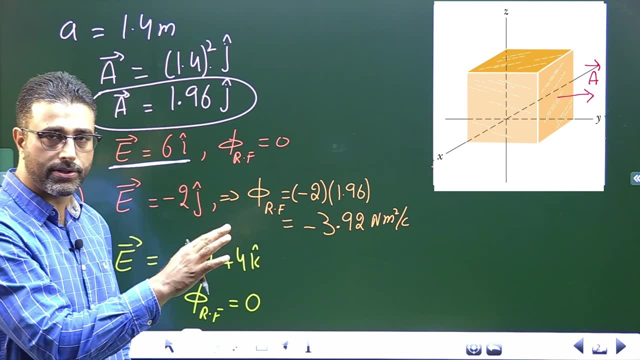 flux through the cube. in all the three cases. well, in all the three cases, field is uniform. 6i. it does not depend on coordinates, okay, so it is constant. this is also constant. this is also constant. so, in all the three cases, field is non-zero. so, in all the three cases, field is non-zero. so in all the 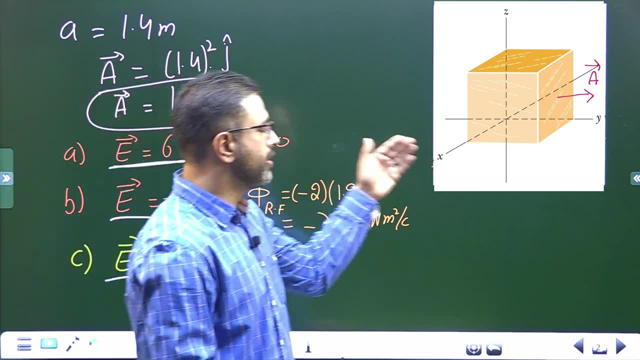 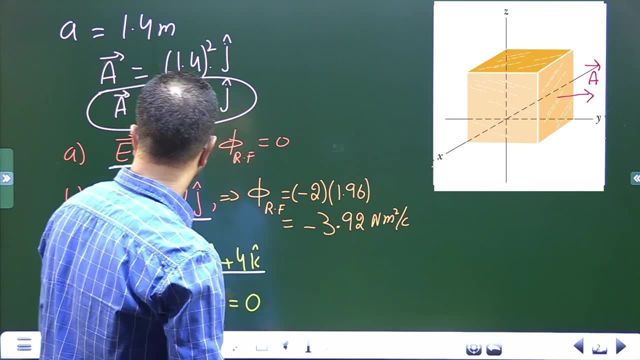 cases, field is non-zero. so in all the three cases, field is non-zero. so in all the three cases, field is uniform. okay, field is uniform. okay, field is uniform. okay, field is uniform. if field is uniform, feel the lines if i draw one of uniform. if field is uniform, feel the lines. if i draw one of the cases. let's say part a, part a, no, let me. 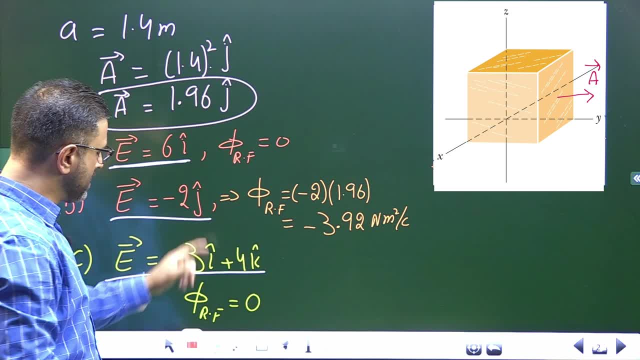 the cases. let's say part a, part a. no, let me draw part b, because part b will be easy there. part b: draw part b, because part b will be easy there. part b: electric field is in negative y direction. okay, electric field is in negative y direction, okay, part b field is in negative y direction. so field is this: 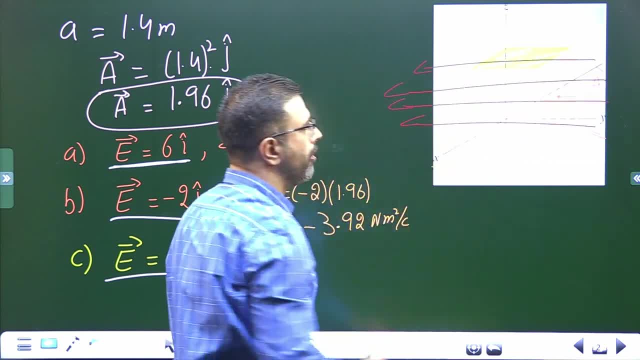 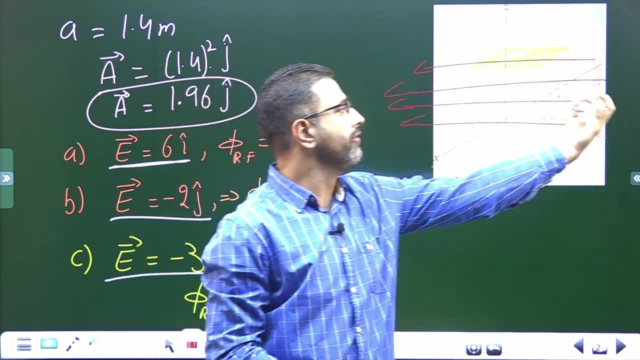 part b, electric field is in negative y direction. okay, part b field is in negative y direction. so field is this way and is a uniform field. so you can clearly see the number of field lines going in is same as number of field lines coming out. So inward flux is same as outward flux. Same will be. 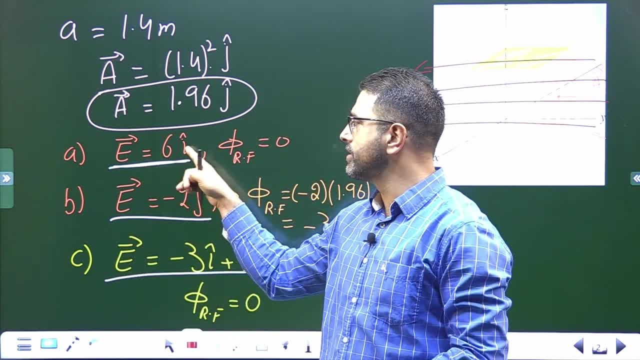 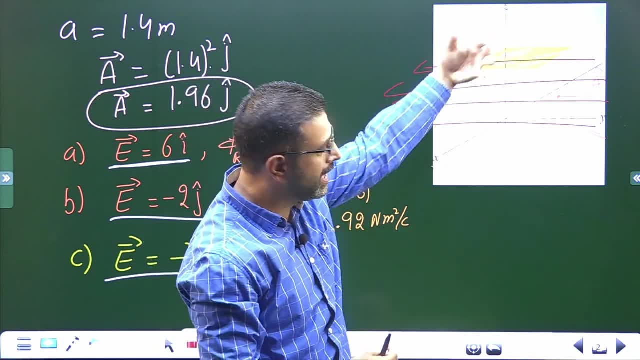 in same will be the case in other cases. Part A: field is in positive, positive x direction. So field is outward. Field is outward. The number of field lines coming in from the back side will be same as number of field lines coming out from the front side, So flux will. 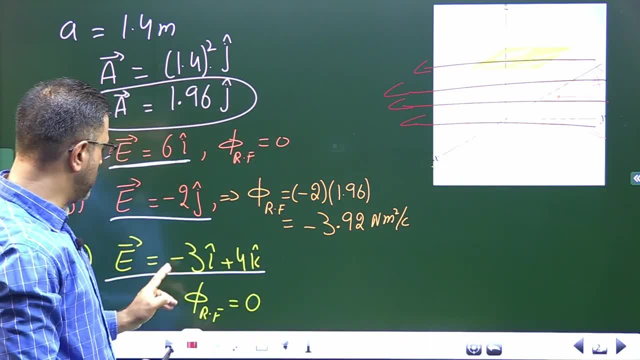 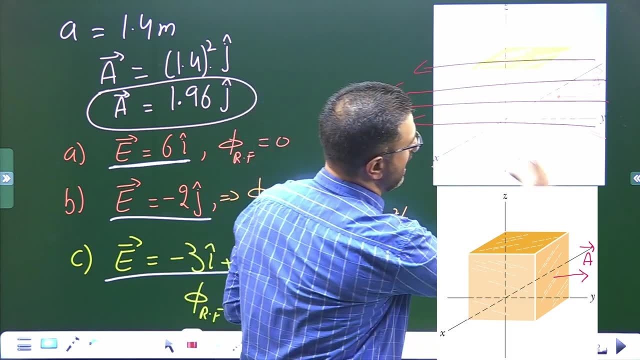 be zero. Okay, Flux will be zero. And then in the third case, field has x component and z component, So field is somewhere here in this direction. So again, number of field lines going in from this side will be same as number of field lines going out from the 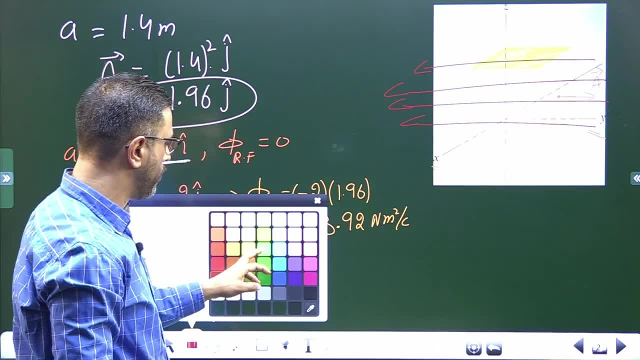 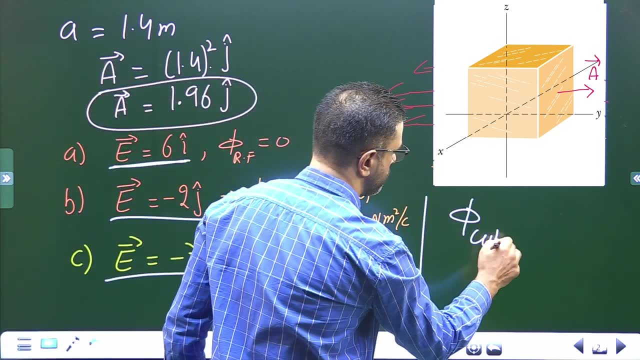 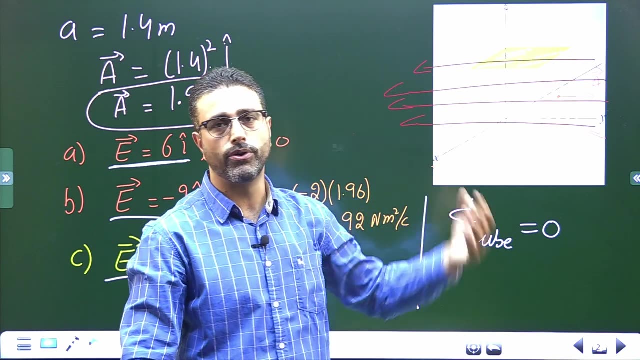 other side. So flux through the closed cube, from for this cube, flux through this cube will be zero in all the three cases. Flux through the cube is zero in all the three cases, Since field is uniform. so flux, inward flux and outward fluxes will be same in all. 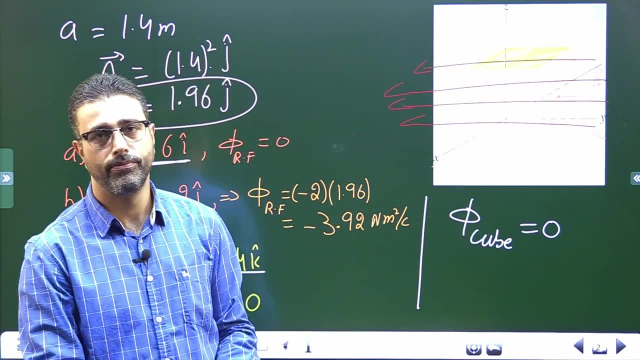 the three cases, So total flux is going to be zero. Okay, That will do for this session.